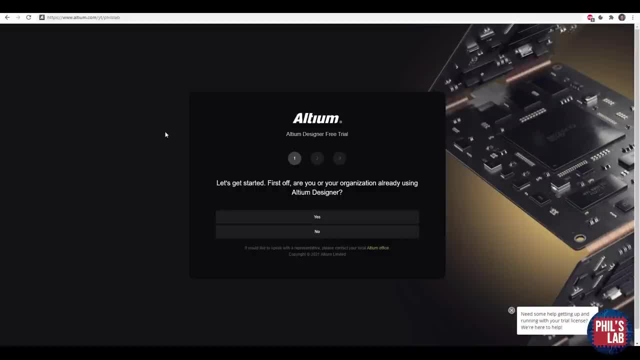 and so forth. Altium is actually offering a free trial of Altium Designer and if you can go to altiumcom slash yt, slash phil's lab, you can get a free trial for yourself to see what Altium Designer is all about. In this first video we'll be covering sensor fusion. 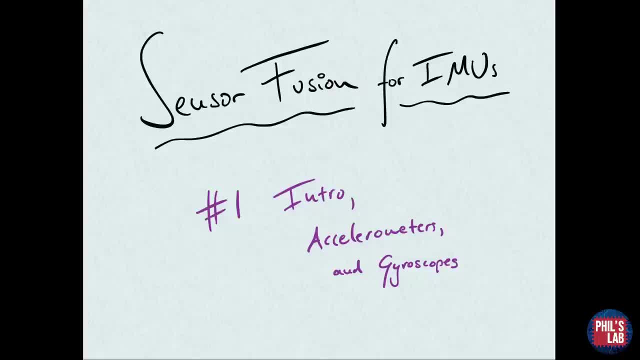 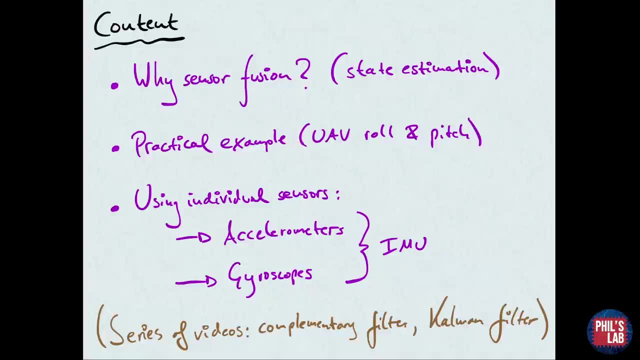 basics and looking at the individual sensors contained in an inertial measurement unit, that is, accelerometers and gyroscopes. We'll look at why we actually need sensor fusion. We'll look at a practical example, which will follow through all these videos, which is estimating the roll and pitch angles for an unmanned aerial vehicle, or UAV for short. 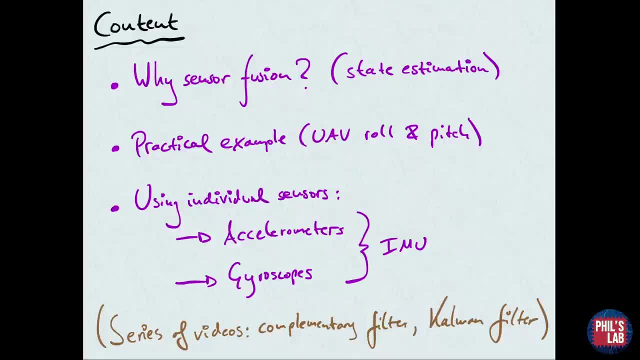 In this video we'll be looking at individual sensors before we'll begin with the fusion part. In particular, we'll be looking at accelerometers and gyroscopes and, combined. these are typically packaged in what's known as an IMU or inertial measurement unit. 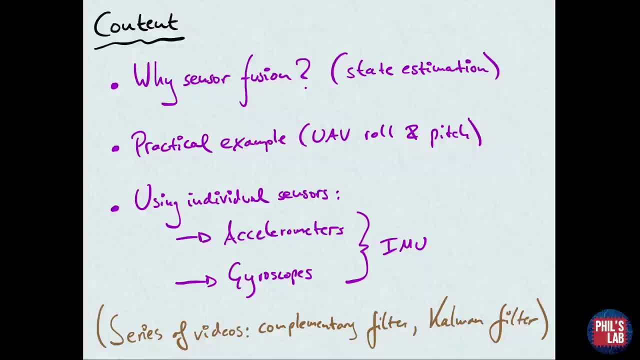 This is a series of videos. the next one will be on complementary filters, which is a very simple sensor fusion technique, and then we'll look at an extended Cowan filter, which is rather more complicated but has better performance than a complementary filter in many. 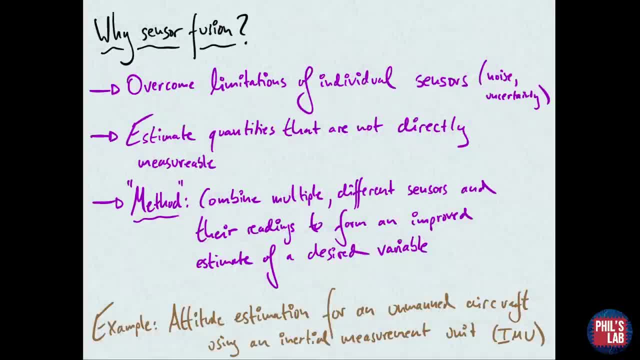 cases. Why do we even need sensor fusion? To keep it short, it overcomes limitations of using individual sensors on their own. in terms of noise, uncertainty and so forth, We can estimate quantities that are not directly measurable. For example, we might have a gyroscope. 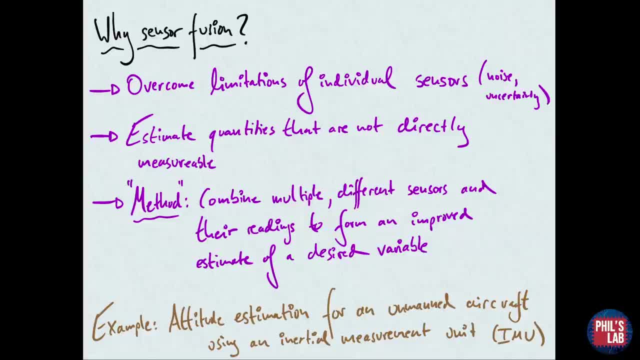 to measure angular rates of change, but we can't directly, with these devices, measure, for example, the roll angle or pitch angle. The method we typically use, and quite simplified, is that we combine multiple different sensors and their readings to form an improved estimate of a desired 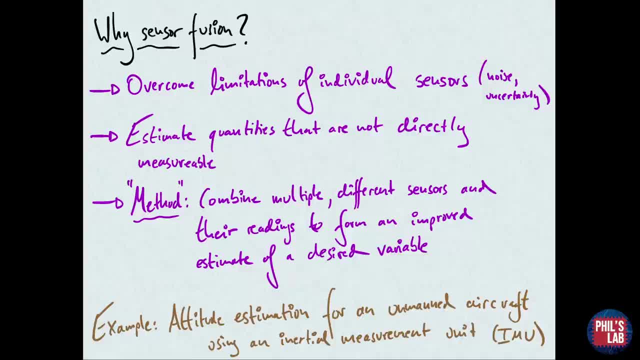 variable, for example, things like roll and pitch angles. The example we'll be using is attitude estimation for an unmanned aircraft using an inertial measurement unit, which, as before, is called IMU for short. Our example is aircraft attitude estimation In particular and in a 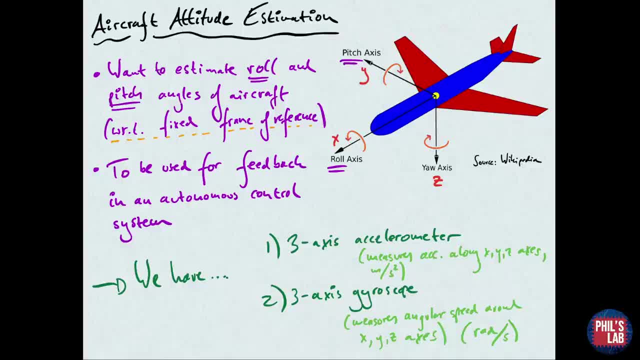 similar case, we would like to estimate the roll and pitch angles of an aircraft, and that's with respect to a fixed frame of reference. So here we see an example of an aircraft and we have the pitch axis, we have the roll axis and the yaw axis, each orthogonal to each other. Now this is: 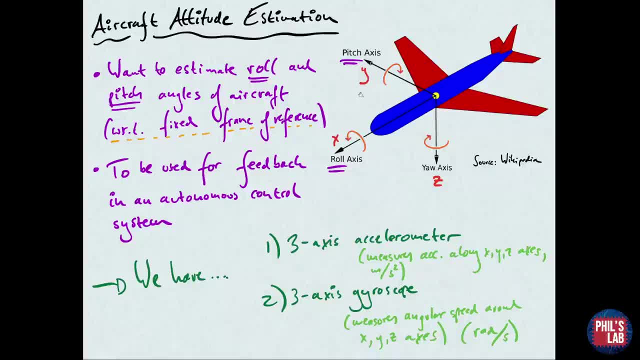 with respect to the body of the aircraft, but we would like it, for example, with respect to a fixed frame of reference, and for simplicity we'll take that as the earth or earth's surface. Now, the reason we might want to have estimates of roll and pitch angles is to be used for feedback in, for example, 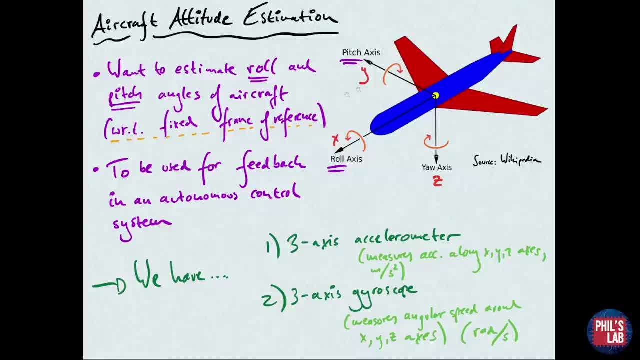 autonomous closed-loop control system. If we have a UAV which is unmanned, we need to somehow autonomously control this, and we need to do that using feedback controllers. Now, in our example, and for many small UAVs, you might only have a limited set of low-cost sensors. In our case, 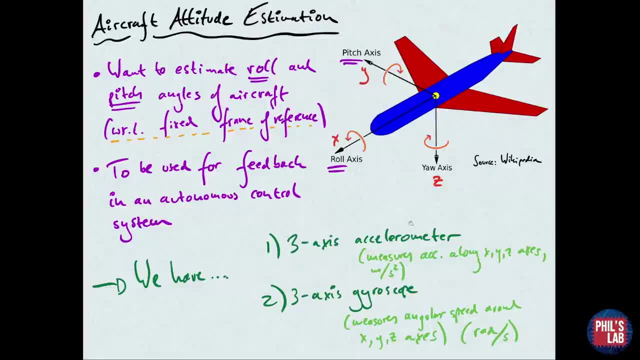 we will have one three-axis accelerometer which measures accelerations along the x, y and z-axis in the body frame, and the units are in meters per second squared. And we also have a three-axis gyroscope that measures angular rotational speeds around the x, y and z-axis. 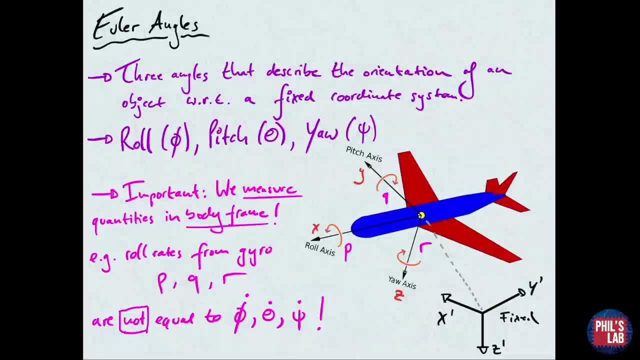 radians per second. Before we start, let's have a brief look at Euler angles, and I won't give a detailed explanation. I will leave links in the description to explain this in further detail. Essentially, Euler angles are three angles that are described with the orientation of an object. 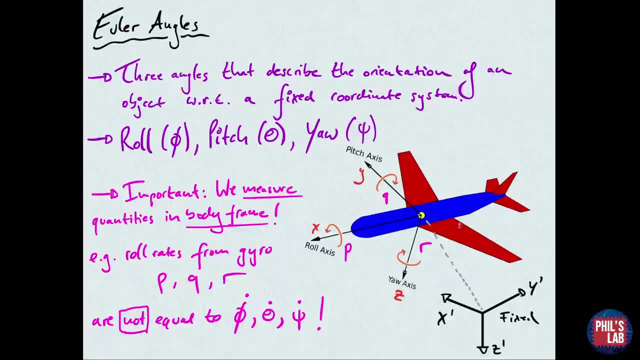 with respect to a fixed coordinate system. So, for example, we have our aircraft here which is pitched, rolled and yawed in its own frame, but that is different to the pitch, roll and yaw with respect, for example, to a fixed frame down here which might be the earth's surface Roll. we 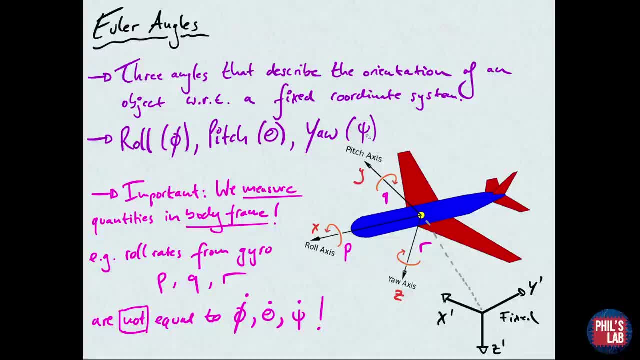 mean pitch by the Greek letter theta and yaw by the Greek letter psi. It is important that we know that we're measuring quantities in the body frame of our aircraft, for example. So the accelerometer and gyroscope measure quantities in the body frame, For example the roll rates from the gyro. 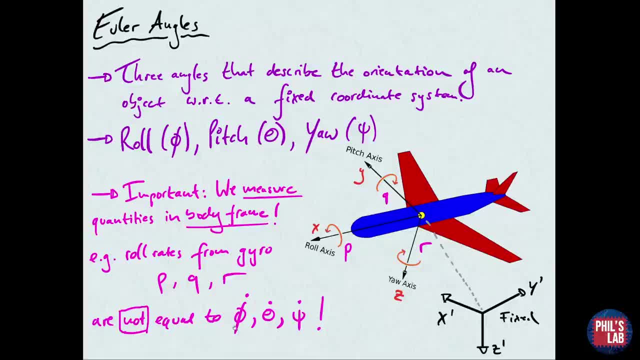 typically denoted by p, q and r, are not typically equal to the Euler roll, pitch and yaw rates which are with respect to a fixed coordinate system. So phi dot, theta dot and psi dot are not necessarily equal to p, q and r, which is what the gyroscope measures, and this will be. 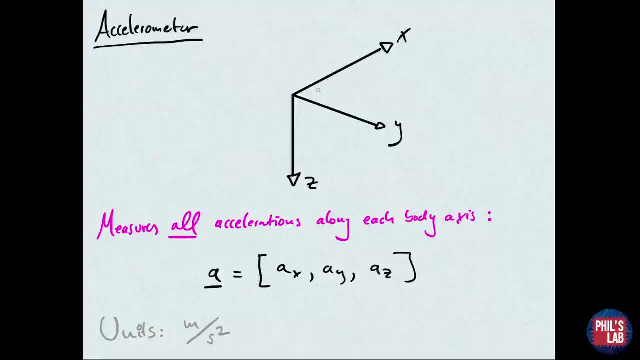 used for the accelerometer. So let's first look at the accelerometer And quite simply, we have our aircraft, axes x, y and z all orthogonal to each other, And our accelerometer is simply placed at the center of our aircraft and measures all accelerations along each body axis. So it'll 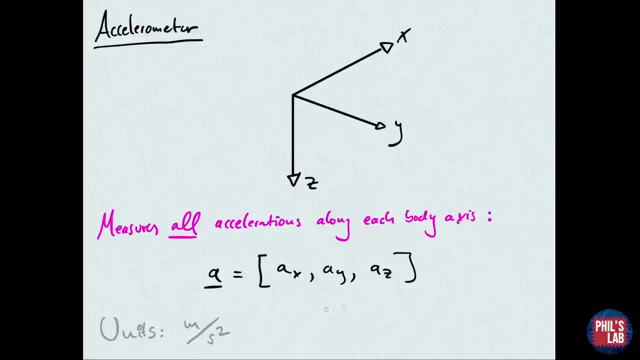 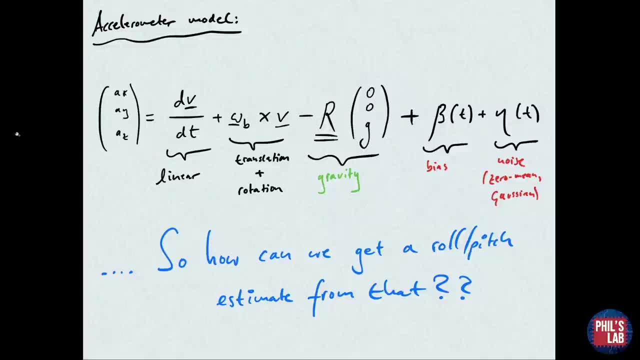 measure it along the x, y and z axes, And we typically have a vector which contains all our measurements And the units are meters per second squared. Now, to be able to use this accelerometer, we have to have an accelerometer model or have an idea of what this accelerometer actually measures. 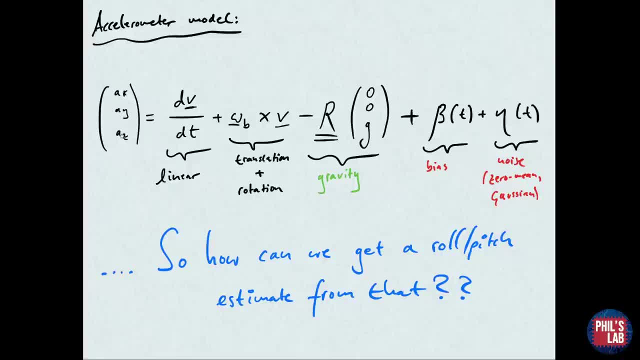 So along the accelerometer, we have the accelerometer and we have the accelerometer and we have the accelerometer. So along this axis, ax, ay and az are measurement terms and that contains our linear accelerations. So dv by dt are accelerations due to translation and rotation, as well as our. 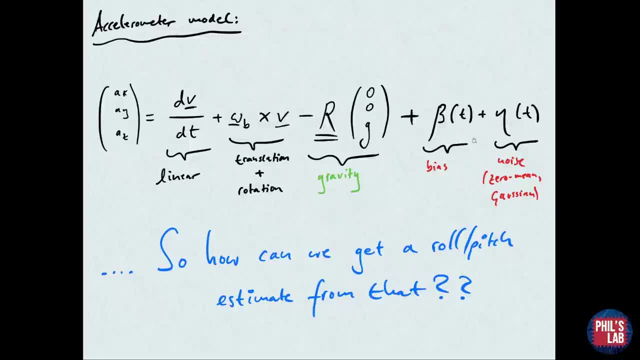 gravity term, But we also have rather unpleasant terms such as a possibly time-varying bias term and a zero mean Gaussian noise term in our model. The question now is: how can we use this accelerometer model in combination with the accelerometer readings to actually get a 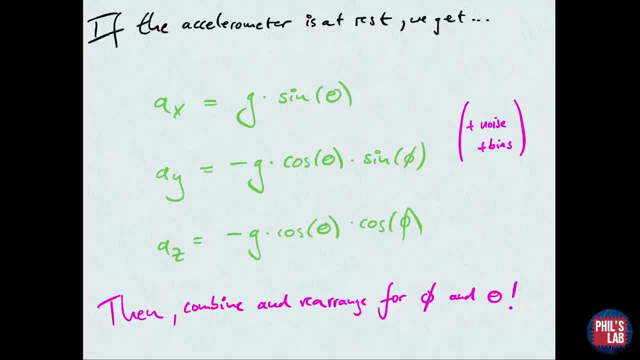 roll and pitch estimate. Now we have to look at a very simplified case to get the answer, and that's if the accelerometer is at rest, So if the translational acceleration is zero, if accelerations due to rotations and translation are zero, And we're pretty. 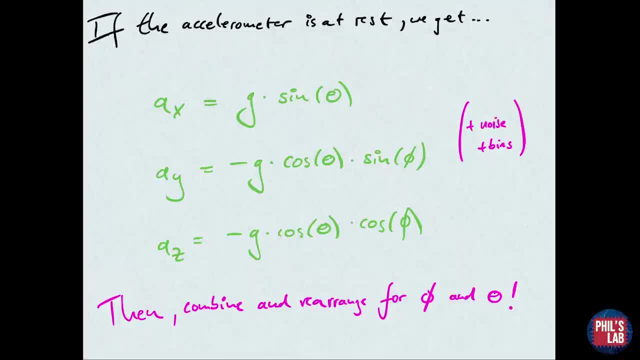 much just looking at the gravity terms and, for the moment, just ignoring the noise and bias terms. Along each axis, x, y and z, we then get these gravity terms. So along the x axis we get g, which is the gravitational constant at the earth's surface. 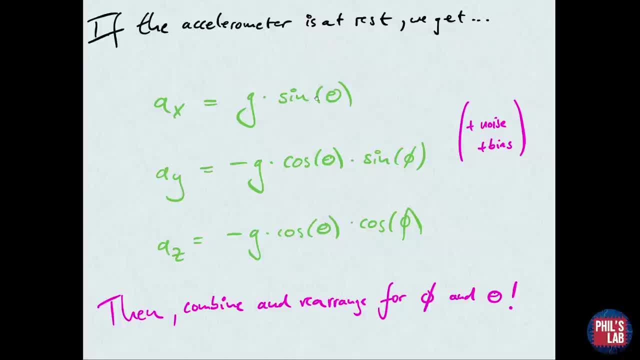 which is 9.81 meters per second, squared times the sine of the pitch angle, And we can go through the y-axis and z-axis terms as well. Now you can see, for example, if we divide ay by az, we get a lot. 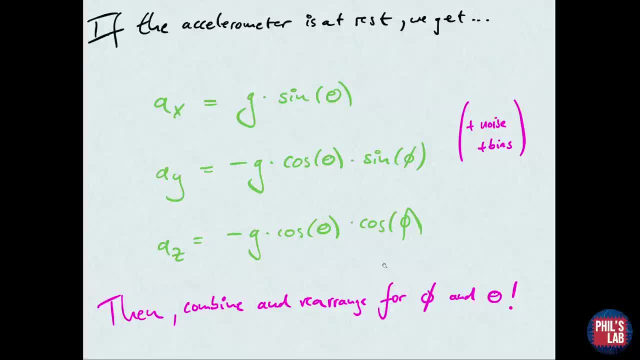 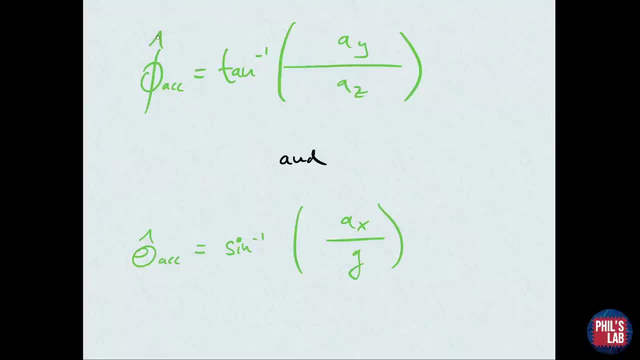 of term cancellations. And this is how we then can find, using just the accelerometer readings, estimates for the roll and pitch angles. So if we simplify and rearrange, notice that this little hat over here indicates that this is an estimate. So phi hat of the accelerometer is our roll. 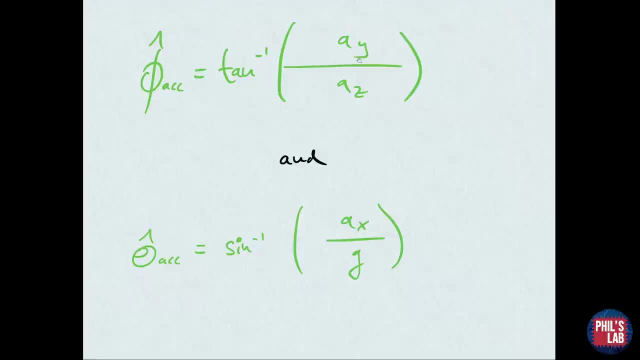 estimate using the accelerometer only, And that's the arctan of ay over az. So, using just the accelerometer measurements And, again, assuming the system is at rest and ignoring noise and bias terms, We can do the same thing for the pitch estimate, and that's the arcsine of ax over g. 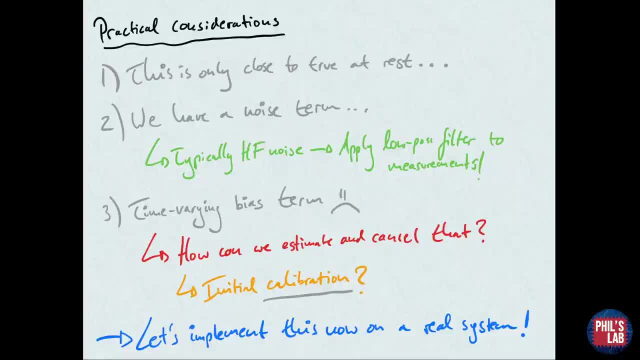 If it were that easy, then we wouldn't need sensor fusion. We have to consider practical implications. Again, this is only close to true at rest, Remember, we have all these other acceleration terms when the accelerometer or the UAV isn't at rest. We also have a noise term. 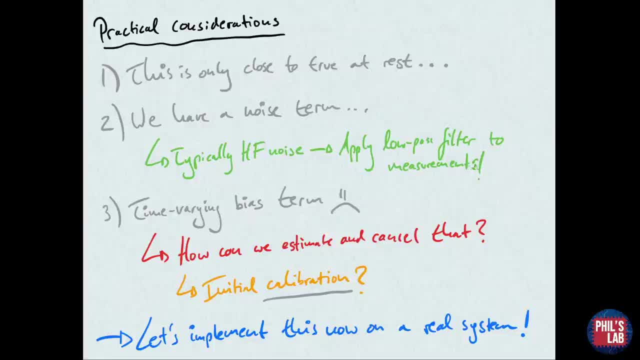 and that is typically high frequency noise, And we can suppress that at least a bit by applying a low-pass filter to our measurement, And that's the way we can do it. So if we have a high-frequency measurements, we also have a time-varying bias term. The question is, can we eliminate that? 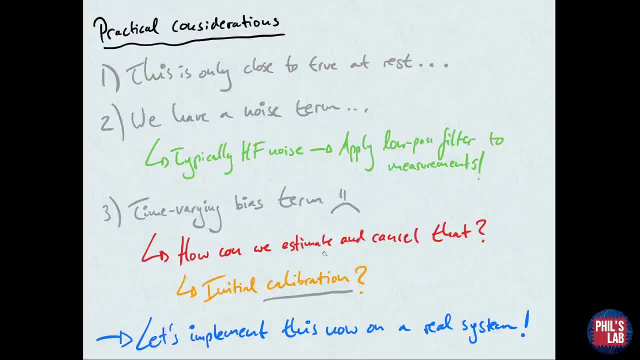 And how can we estimate that We can do an initial bias elimination? by doing an initial calibration of the sensor, So keeping the sensor at rest and then averaging some readings and then estimating our bias. But let's have a look first and implement this on a real system. 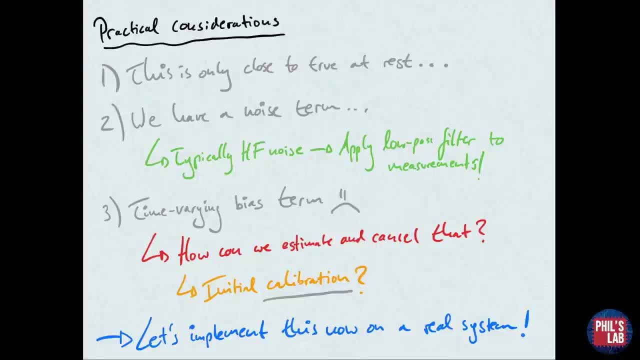 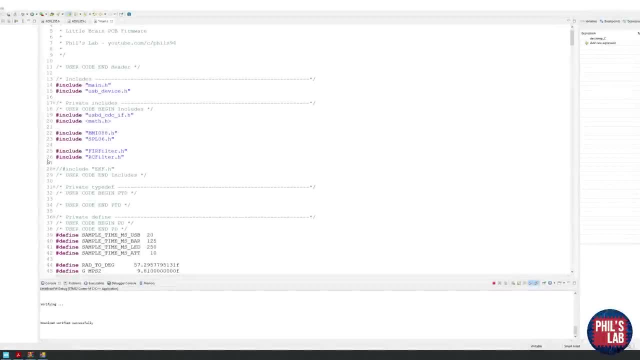 on an STM32-based embedded system to see if this actually works and when it doesn't work. So here we are on STM32-cube-IDE, and I have opened my LittleBrain firmware, which you can find in my GitHub repository, And this has basically set up all the drivers for the IMU to read the raw values. 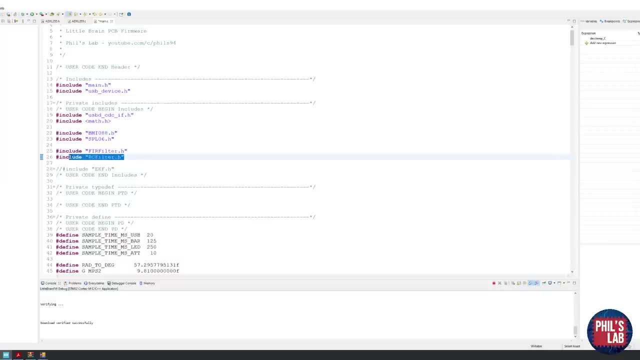 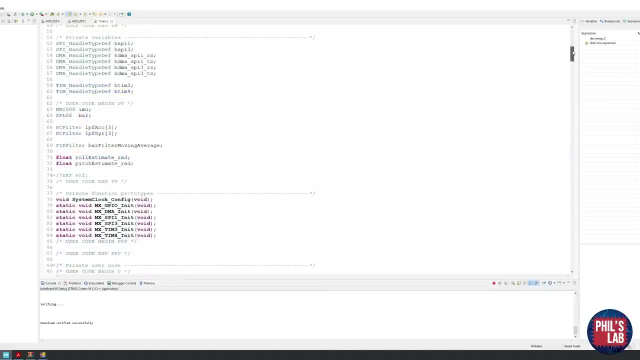 for the accelerometer and gyroscope, as well as an RC, simple IRR first-order low-pass filter implementation to filter my raw accelerometer and gyroscope readings. I'm reading my accelerometer and gyroscope values via DMA and then filtering them In my main routine. I will then get the. 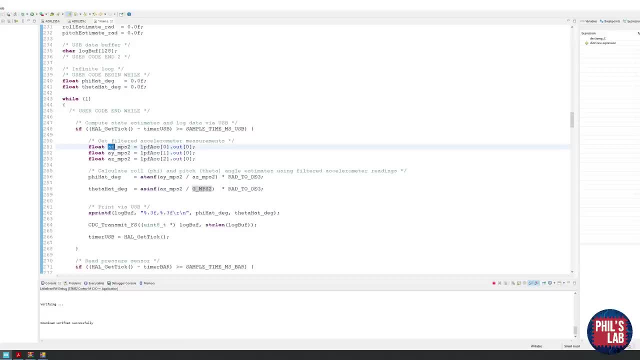 filtered accelerometer measurements which I read out by DMA, So AX in meters per second, AY in AZ, all in meters per second squared. Then I will calculate my roll and pitch angles, that is, phi and theta, using the filtered accelerometer readings. 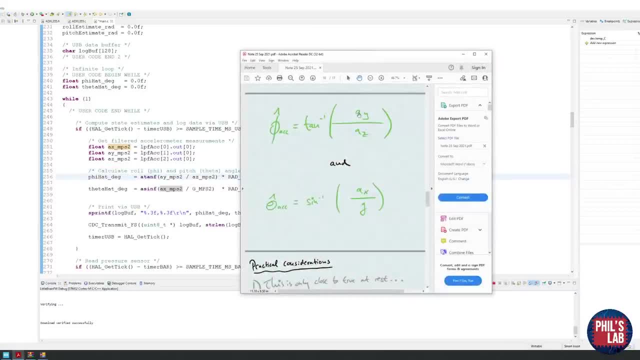 Now, if you remember from the slides, for the roll angle, that's the arctan of AY over AZ, and for theta, which is the pitch angle, that's the arcsine of AX over G, And that's exactly what. 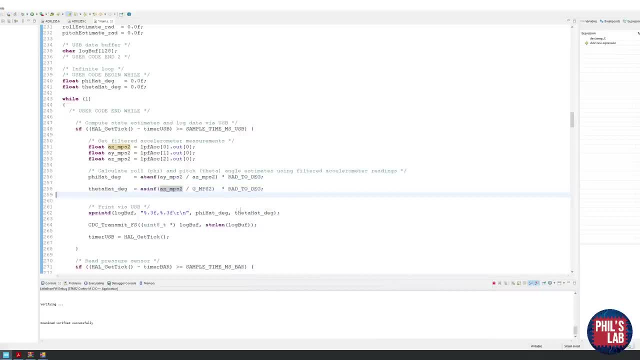 I've done here and here. Then I print the resulting angle estimates via USB and the virtual comp port. Now this program is already compiled and running on my LittleBrain board, So let's switch over to the serial oscilloscope which plots my 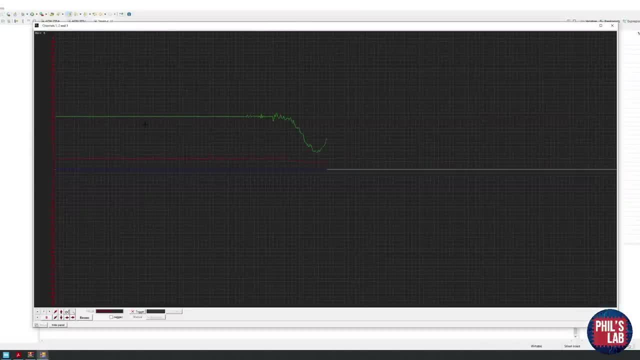 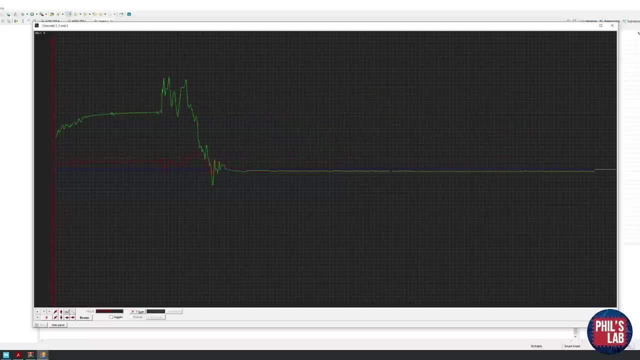 incoming virtual comp port data. Now I have the LittleBrain board on my one hand and you can see the green trace is my roll angle and the red trace is my pitch angle. From this point onwards, I have my LittleBrain board flat on the table, flat on my desk, As you can see the estimates. 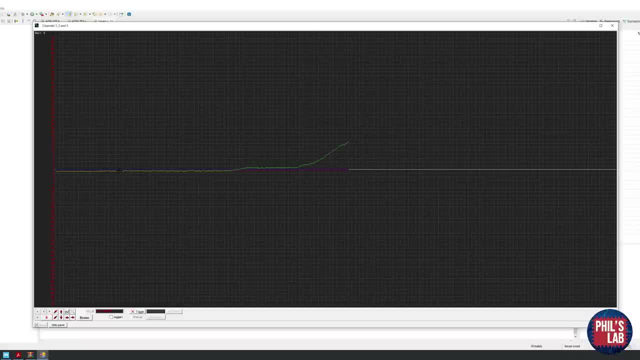 are pretty much okay, pretty much zero degrees. Now, as I start rolling my board very, very slowly, you can see that roll angle increase, decrease as I'm rotating my board. So I'm trying to do it as slowly as possible as to not introduce any extra acceleration. 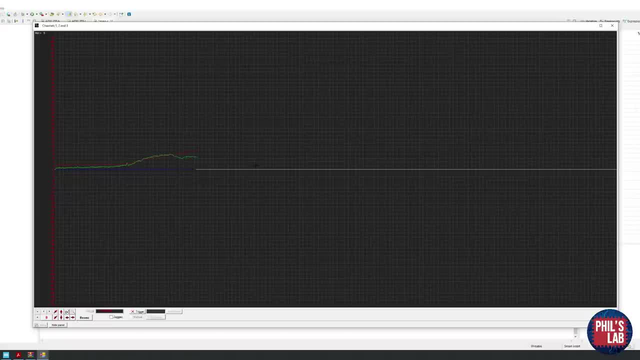 I can do the same thing with my pitch angle. I'm trying to move the board up slowly. As you can see, my accelerometer roll estimate is also changing, And this is because of many of these non-idealities. I can't keep the board perfectly unaccelerated, and that's why I'm getting errors in my readings. 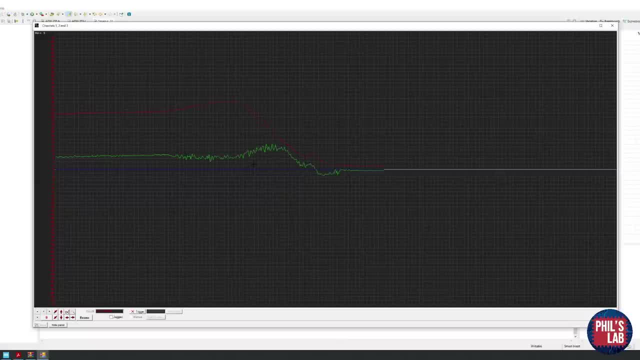 Now, if I keep my board flat again on the table and then just yaw the board so I'm not rolling or pitching at all, you can see I'm actually getting changes in my roll and pitch angles just by yawing, And this is because 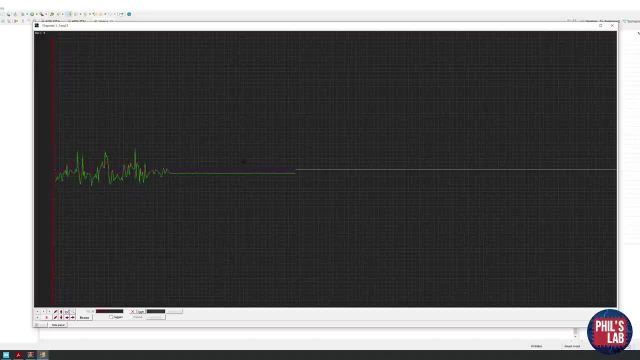 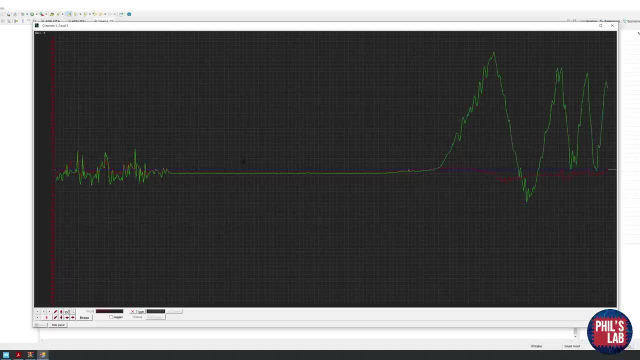 of all these extra acceleration terms that we haven't accounted for in our model and in our estimate of our roll and pitch angles. Also, if I roll my board rather quickly, you can see it's not ideal as well. The pitch estimate is also varying quite a bit, So this: 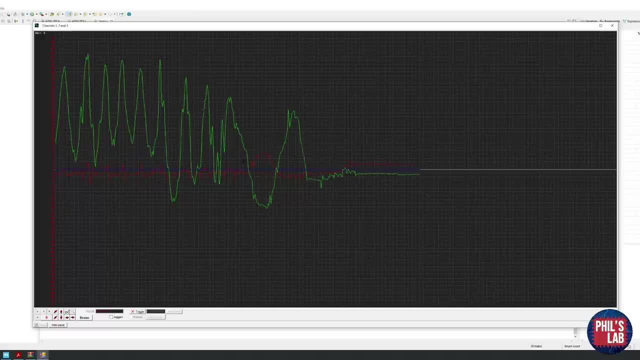 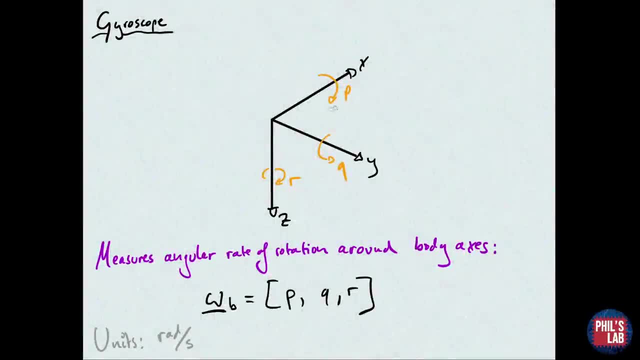 isn't entirely ideal. It's okay when we're not accelerating very much and then the board is fairly at rest, But other than that it's not that great. So now let's look at the gyroscope Again. we have our body frame axes, so X, Y and Z. 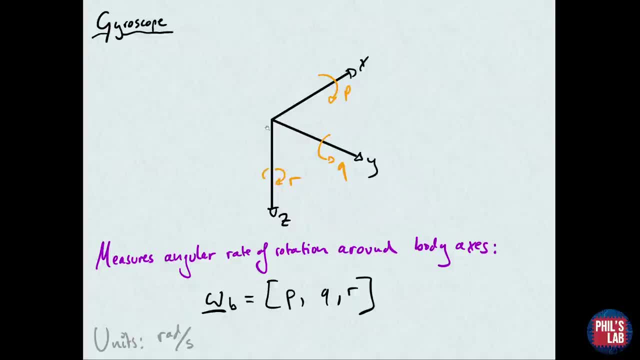 And our gyroscope measures the angular rate of rotation around the body axes. So how fast, essentially, around each axis, does our system rotate? Around the X axis, we denote this by P. along the Y axis, we denote this by Q, and around the Z axis, we denote this by R And we can form: 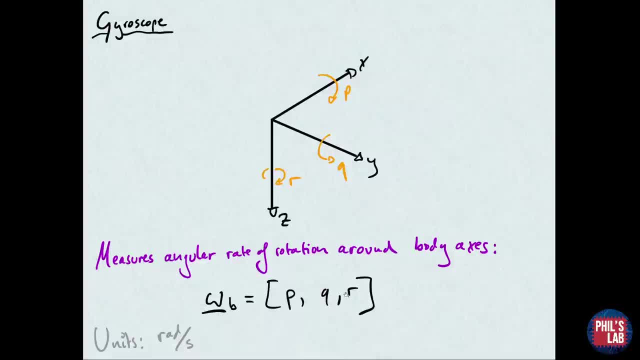 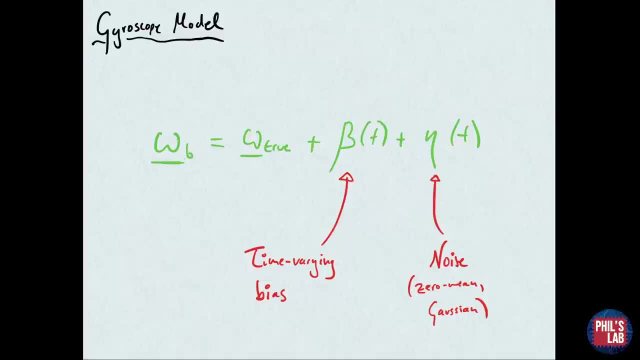 a vector which is an omega, and the body frame is composed of P, Q and R, And the units are in radians per second. Now, our gyroscope model is quite a bit simpler than the accelerometer model. Essentially, what we measure is our true angular acceleration. 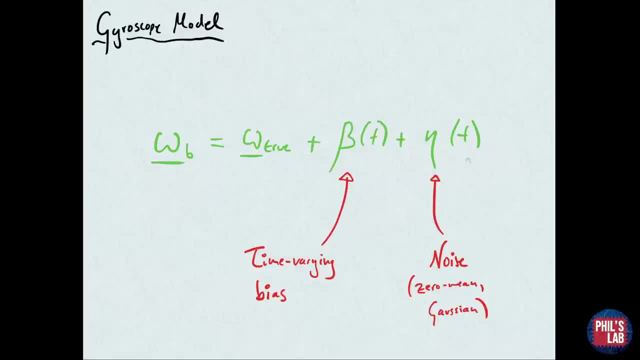 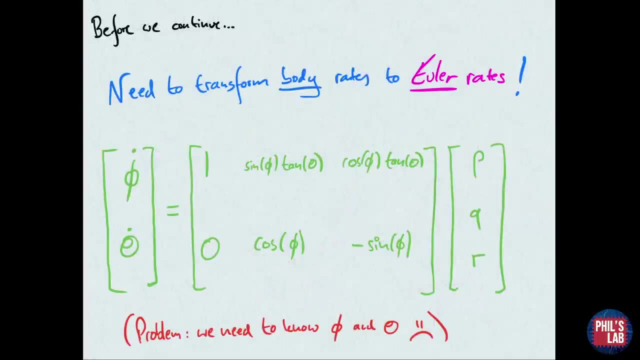 some sort of time-varying bias which will become important later, And again, some noise term which is typically modeled as zero mean Gaussian noise. Now, coming back to our Euler angles, we need to remember that we need to transform the body rates, which are P, Q and R, to Euler rates. 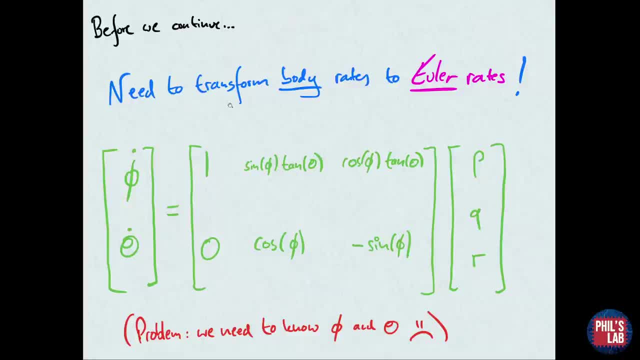 which are phi dot, theta dot and psi dot, And the way we do this is via this matrix, here, for example. So P, Q and R multiplied by this matrix gives us our angular rates of change in the Euler, or fixed inertia. 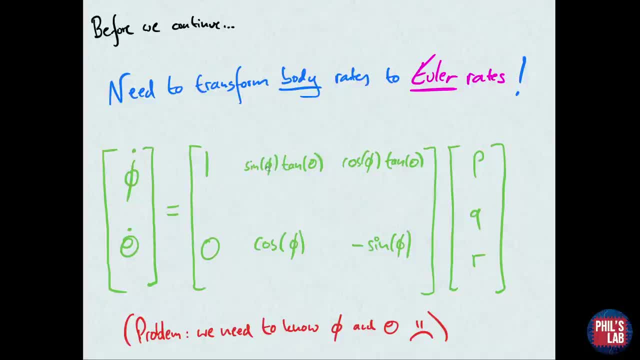 Now, as you can see here, this again depends on phi and theta already, So that can be a problem. We actually need to know phi and theta to get our measurement vector P, Q and R from our gyroscope into our inertial frame. Can't we then simply integrate our Euler rates, phi dot and theta dot? 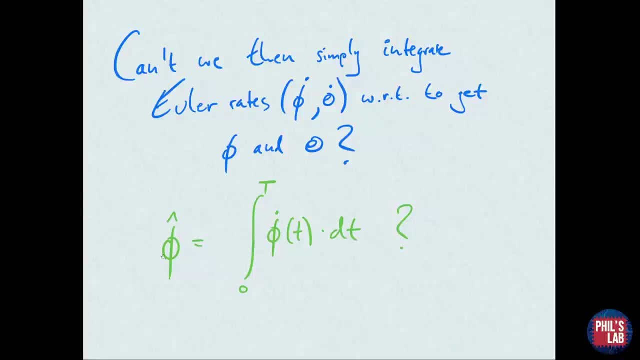 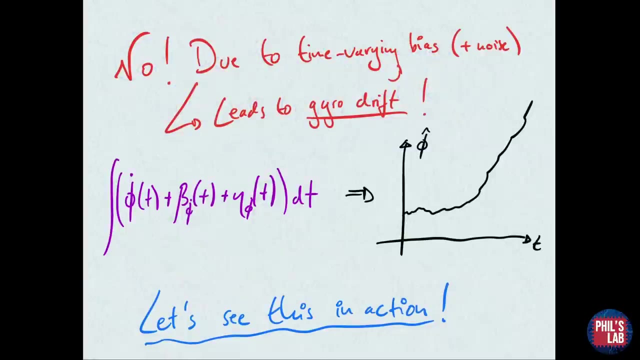 with respect to time to get phi and theta. So, for example, this integral here, our estimate of the roll angle, could just simply be the time integral of our Euler rates, which we can get almost directly from our gyroscope. And the non-idealities of our sensor make this pretty much impossible, And this is mainly due to 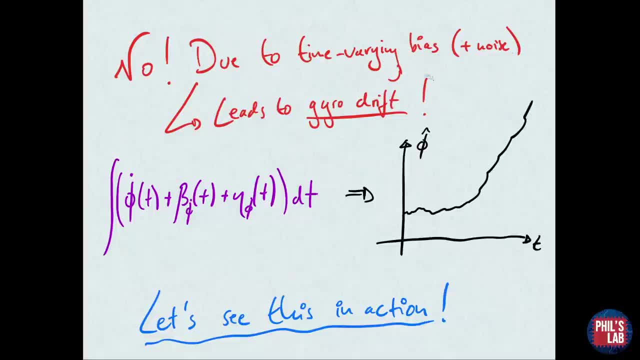 our time varying bias and, of course, the noise term, And this is typically what needs to gyro drift because of this time varying bias. If we integrate the actual measurement, so we get our theta dot but we also have a bias term and noise term. If we integrate that, the gyro estimate of 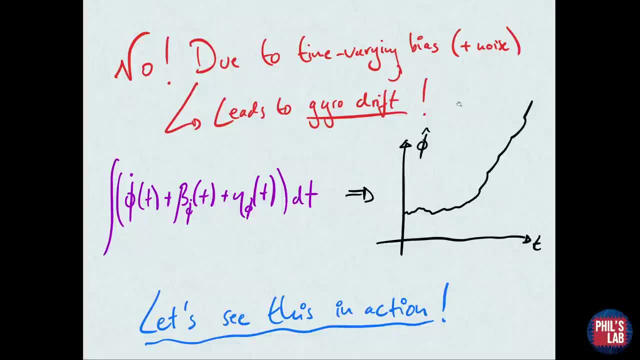 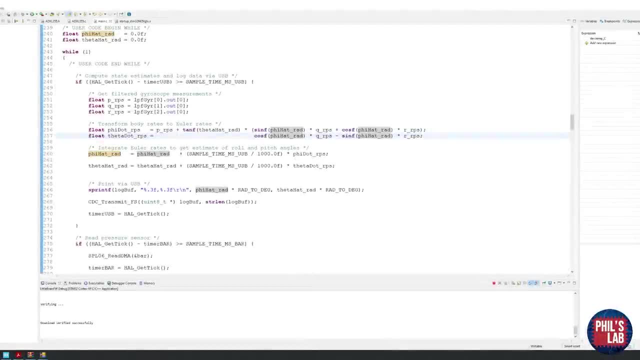 the angle actually drift away, and rather quickly, so for very inexpensive gyros, But let's actually see this gyro drift in action. So now let's look at just the gyroscope implementation of trying to estimate our roll and pitch angles. I have my initial angle estimates, which I'll just set to zero, and this is for roll. 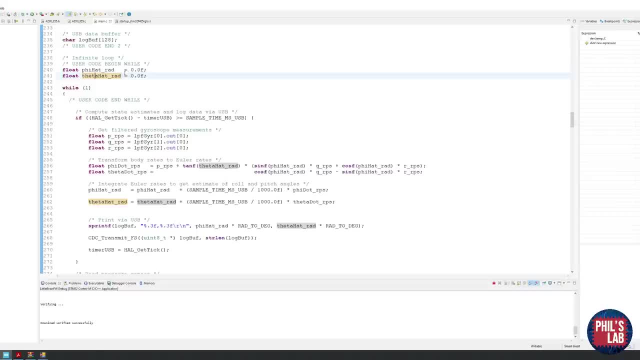 and pitch and I'll set them both to zero radians. I'm working radians and then I'll convert it to degrees. So at a fixed sample rate I will get my filtered gyroscope measurements, which are called P, Q and R, all in the units of radians per second. Then I will transform my body rates to. 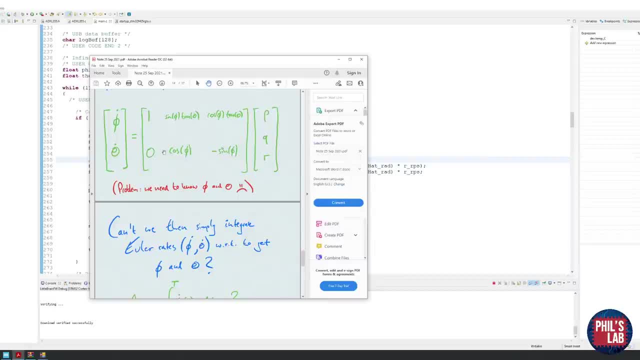 Euler rates. Again, looking at the slides, this is simply doing this: matrix times, R measurement vector, So P, Q, R times. this gives me phi dot and theta dot, So Euler rates versus these body rates. over here I need to know my theta estimates and phi estimates to be able. 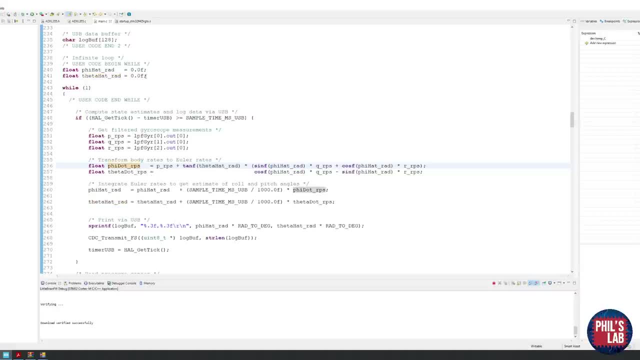 to compute these Euler rates. So this is a bit problematic because we are basing this all on estimates as before. Now, once we have these Euler rates, we can integrate them with respect to time to get estimates of roll and pitch angles, And I'm doing that via simple Euler. 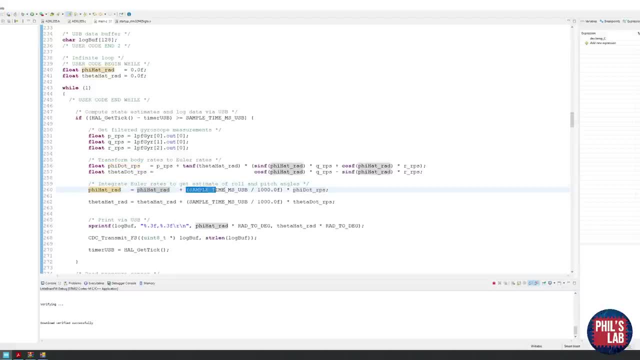 integration. So the new estimate is the old plus DT, which is the sample time in seconds times the rate of change. This is a simple numerical integration and I'm doing that for the roll estimate and the pitch estimate. And then I'm converting these measurements in radians to: 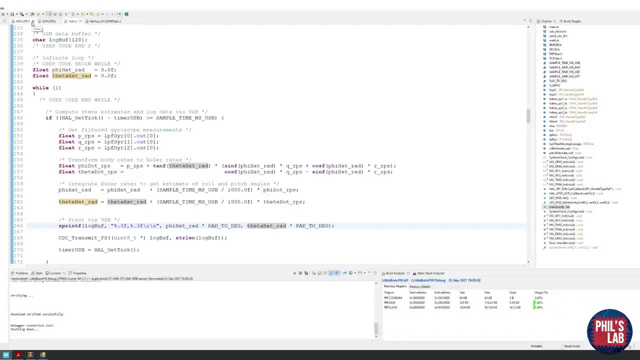 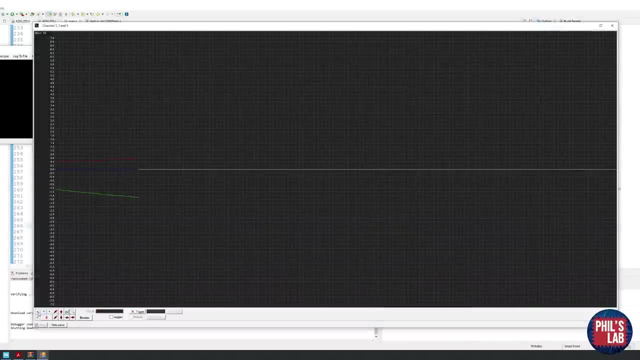 degrees and sending them over via USB. Let me just upload this code to the board, Then I'll open my serial oscilloscope and connect. I have my board flat on the table. at the moment. I am doing nothing to the board. As you can see, these pitch and roll estimates are diverging from where they 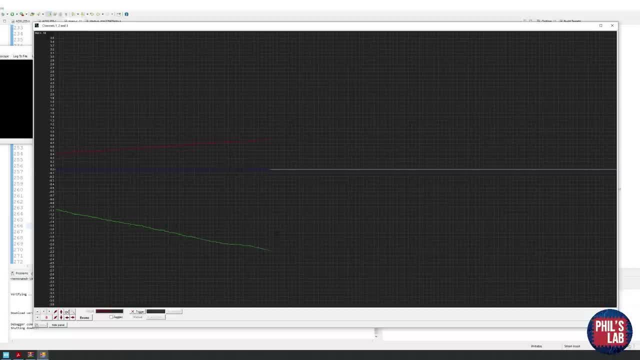 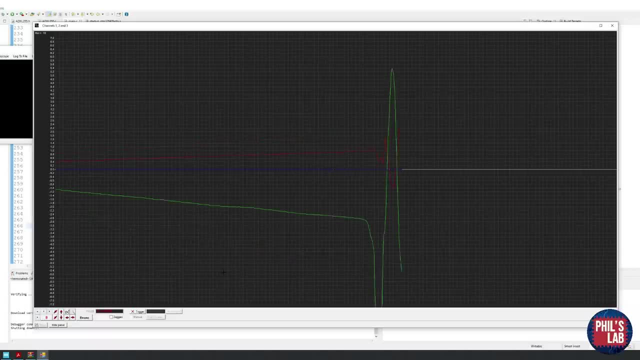 should be. They should be at zero, but because of our time, varying bias and noise terms, we are integrating these areas and we're drifting away from our true value. Now I can rotate and pitch and roll my board. That's all completely fine, But 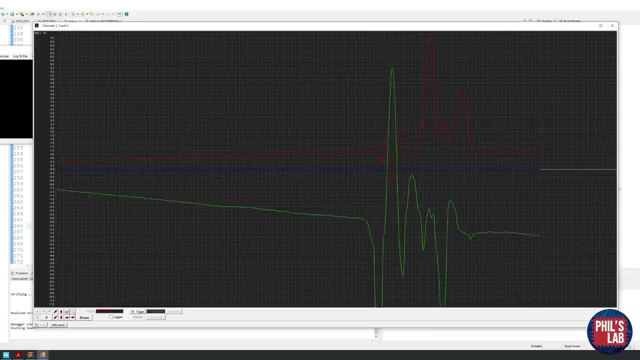 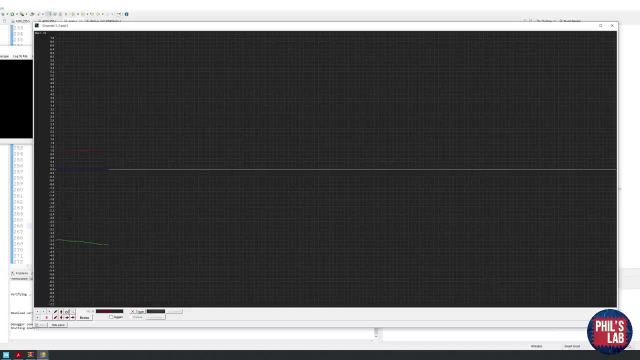 at steady state. if I have my board flat on the table again, you can see the angle is not where it should be. It should be both at zero. Pitch and roll should be zero, but they are very, very quickly diverging from their true state And this is called gyro drift and it's a real problem if 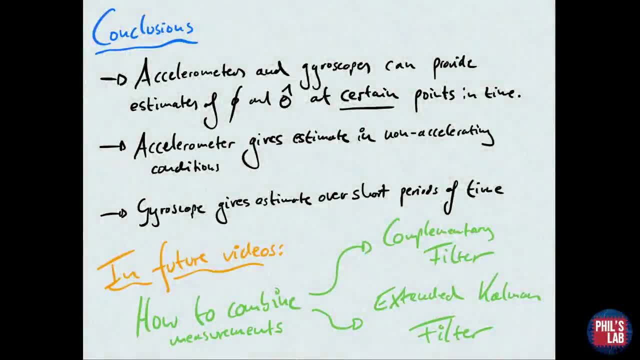 we're just using gyroscopes on their own. Now that we've seen both the accelerometer problems and gyroscope problems- when we're using these sensors individually to estimate our roll and pitch angles- we can draw some conclusions. Now accelerometers and gyroscopes can actually provide estimates of phi and theta- our roll and pitch. 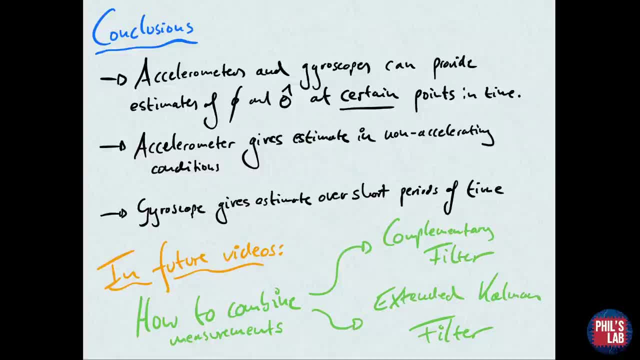 angles at certain points in time, meaning that accelerometers give an estimate in, for example, non-accelerating conditions and gyroscopes give estimates over shorter periods of time, for example, But accelerometers have problems when they are in accelerating motion Gyroscopes. 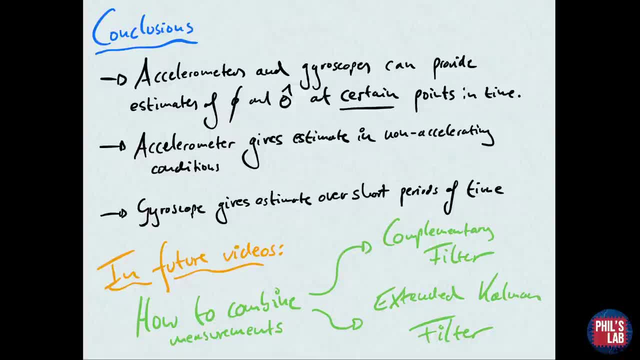 on the other hand, have a rather annoying bias term which leads to bias drift if we simply measure them. In future videos I'll show you how to combine these measurements of the accelerometers and gyroscopes using two different methods. One is really simple, called the complementary filter. 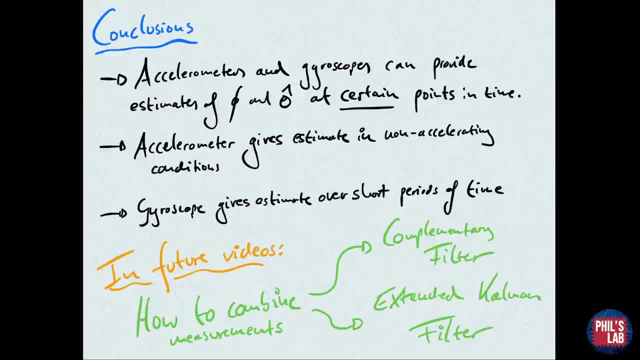 and is very simple and efficient to implement, but doesn't always give the best results. A typically much better way of implementing sensor fusion is via what's known as a Kalman filter, and we'll be looking at the non-linear variant called the extended Kalman filter in a future video. Thanks again for watching and I hope to see you in the next video.